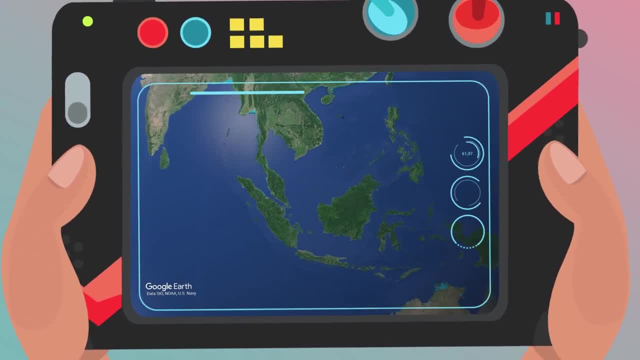 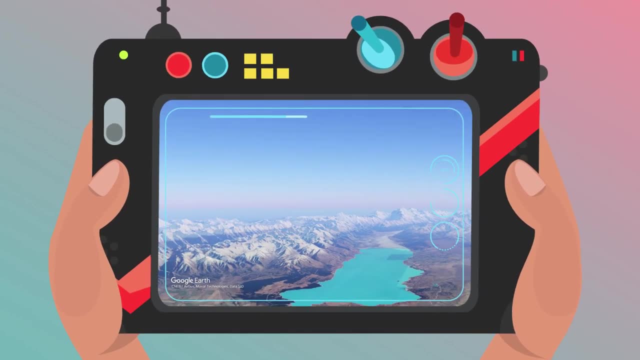 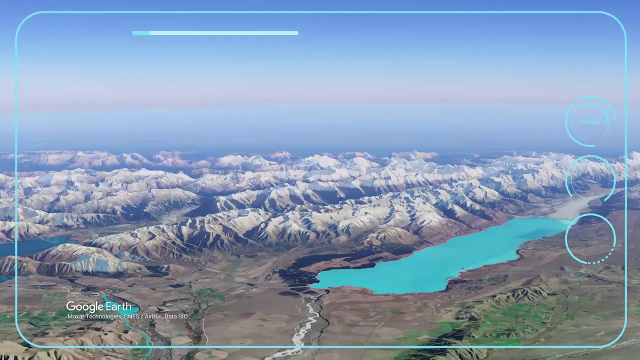 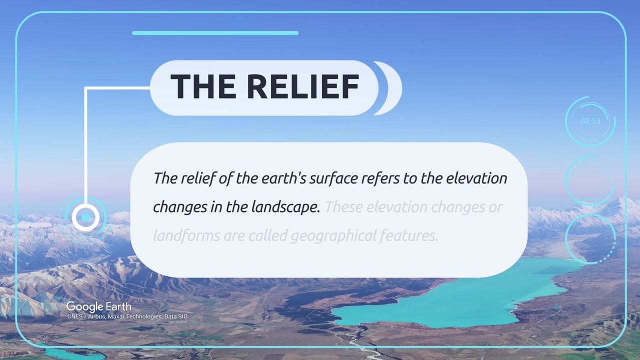 brown and green landmasses that make up the scenery. From up here I can see that the surface of the Earth is shaped differently. This must be the relief of its surface. The relief of the Earth's surface refers to the elevation changes in the landscape. These elevation 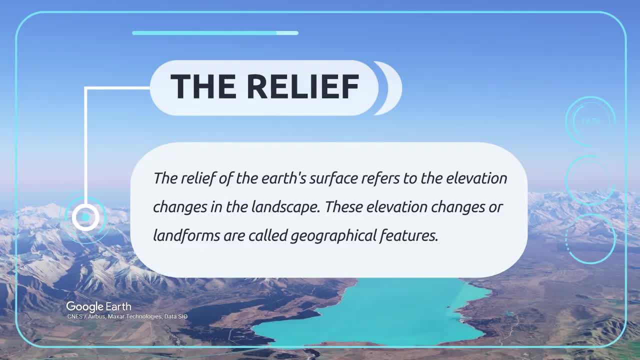 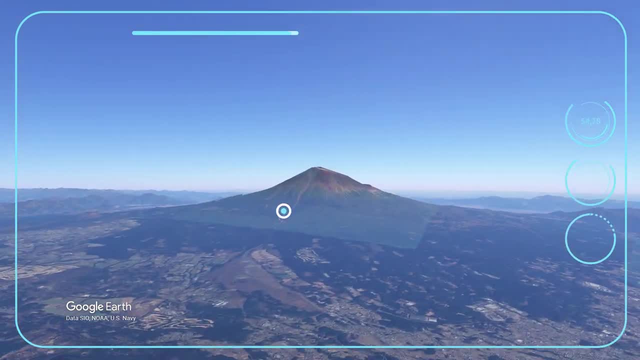 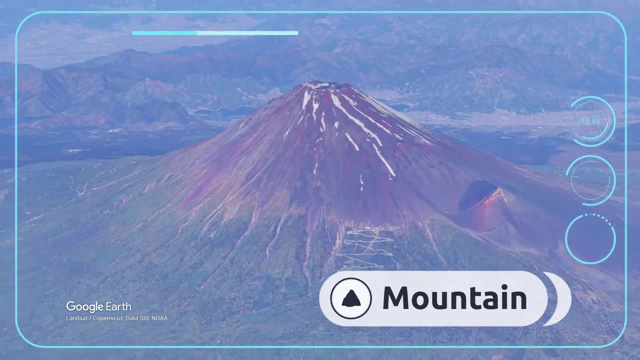 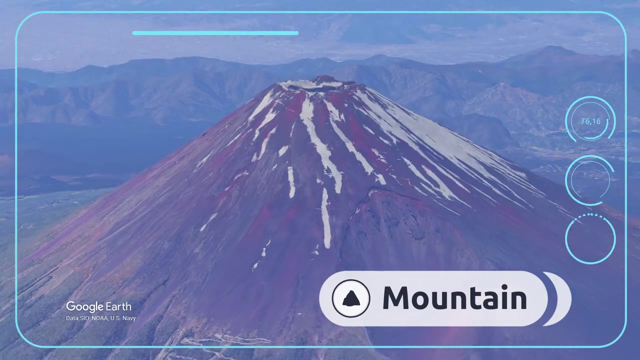 changes or landforms are called geographical features. What are geographical features? Deposits and locations? Mountains: A mountain is a land mass which may also be made up of blocks of rock that rise above its surroundings. Mount Fuji is in Japan. Mountains: 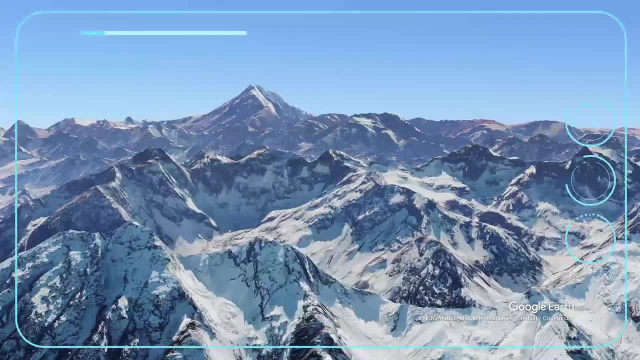 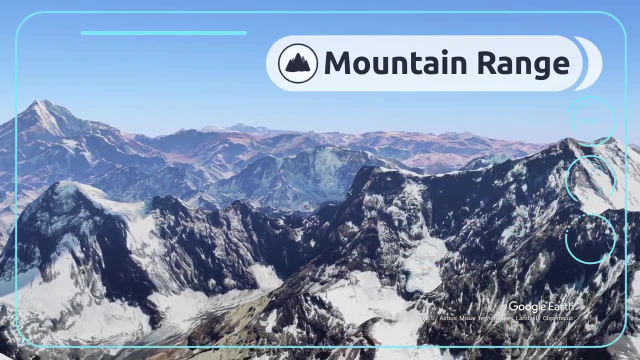 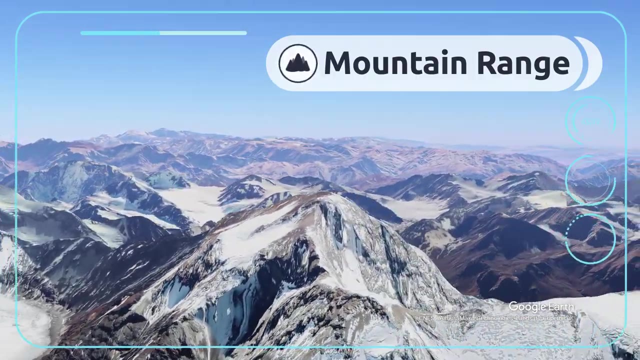 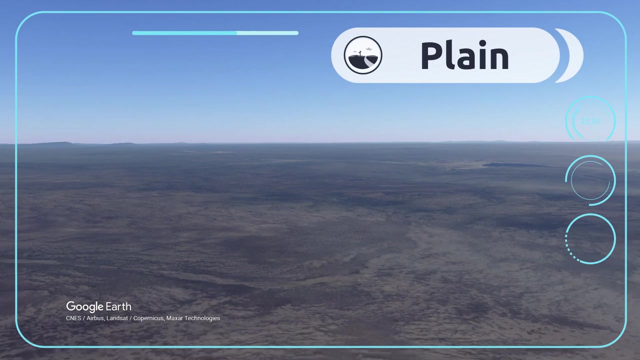 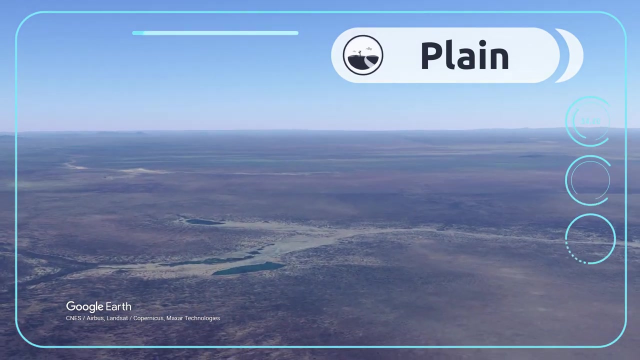 Mountain range. A mountain range is a series, series of mountains connected together. I can see the Andes mountain range from up here. Mountain Range Plains- Plains are vast areas of flat land that stretch across the Earth's surface above sea level, For example, the Serengeti Plains in Africa. 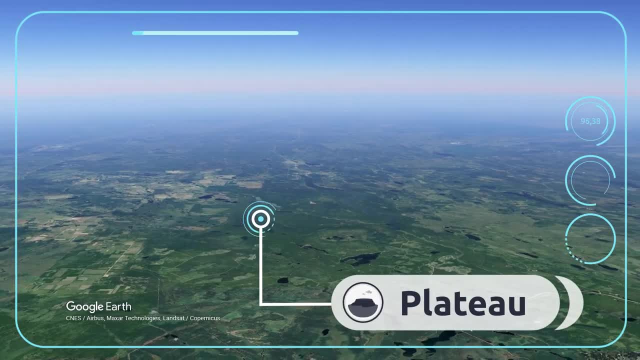 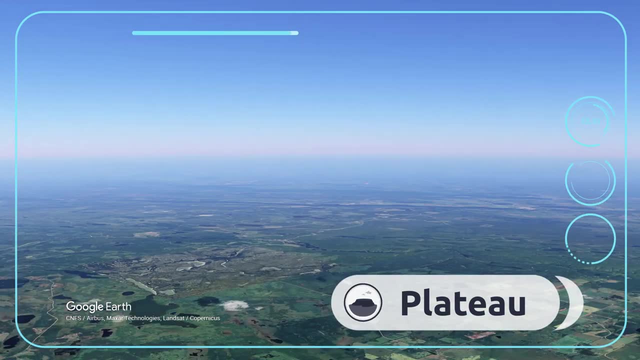 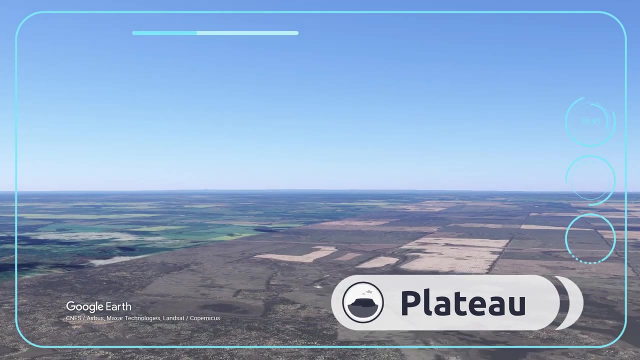 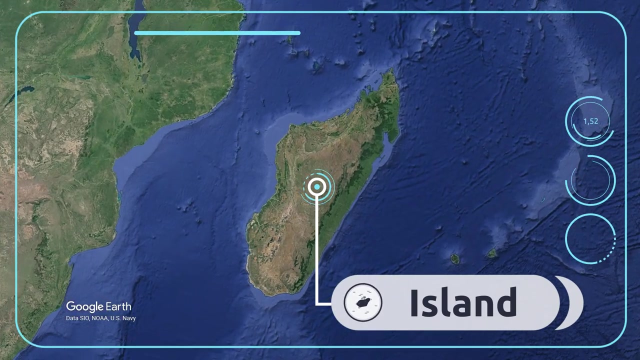 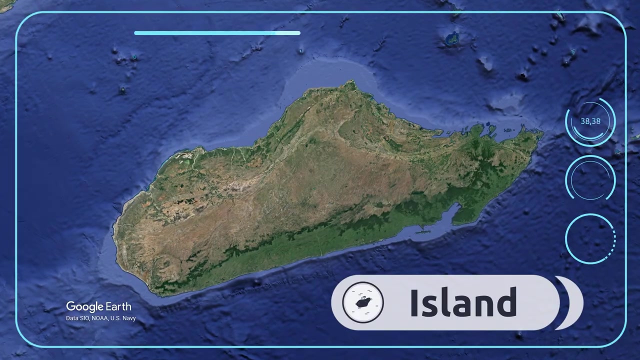 Plains Plateau. A plateau is a flat area of land high above sea level. Look, this is the Missouri Plateau in North America. Plateau Island, An island, is a tract of land surrounded by water. Look, right there, it's the island of Madagascar in Africa. 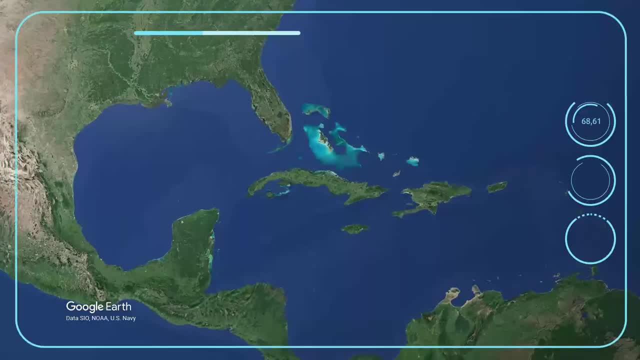 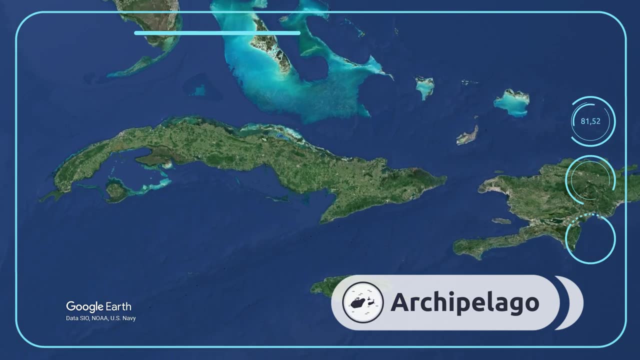 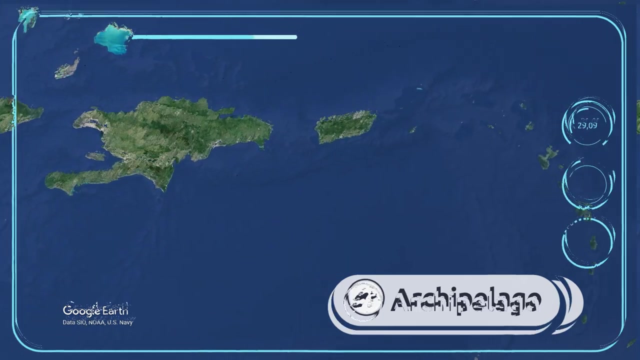 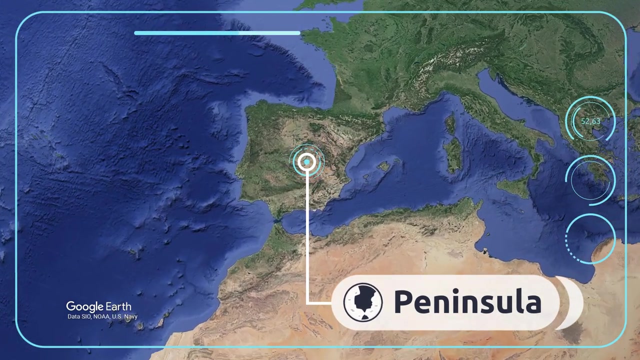 Island Beech Archeopelago. An archipelago is a group of many closely scattered islands, for example, the Caribbean archipelago between North and South America Archipelago Peninsula. A peninsula is a portion of land surrounded by water on three sides. 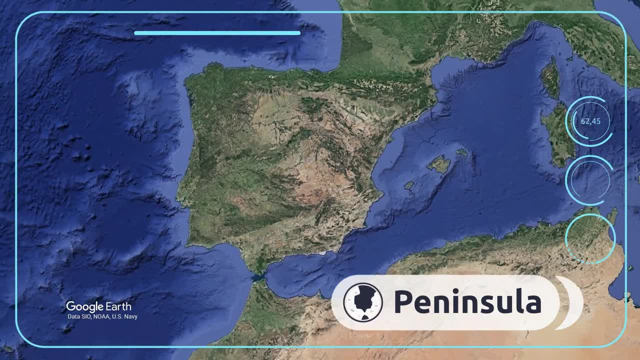 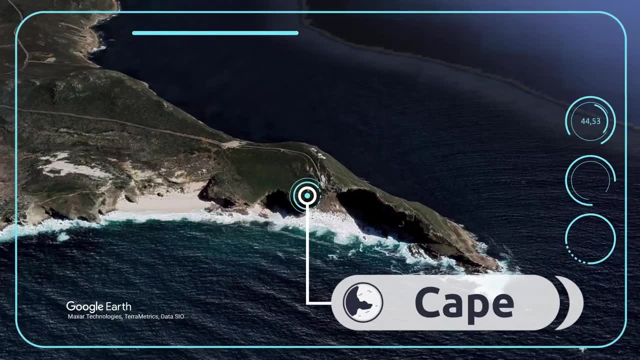 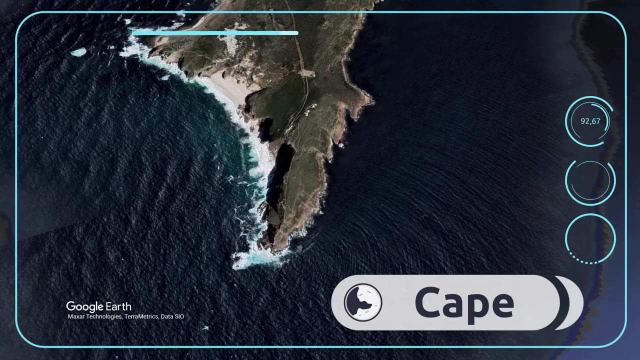 Can you name a peninsula? That's it: The Wonk, Iberian Peninsula. Peninsula Cape: A cape is a narrow part of land that extends into the water, usually the sea. The Cape of Good Hope is one of the most famous capes in the world. 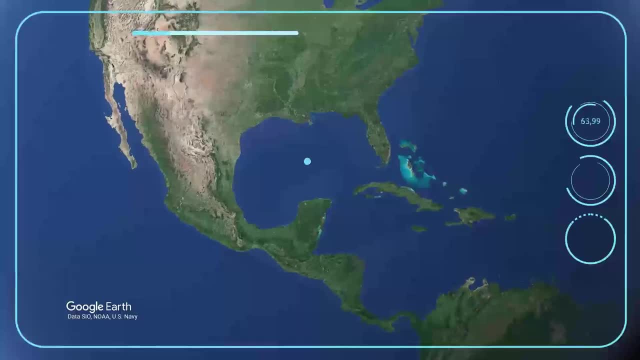 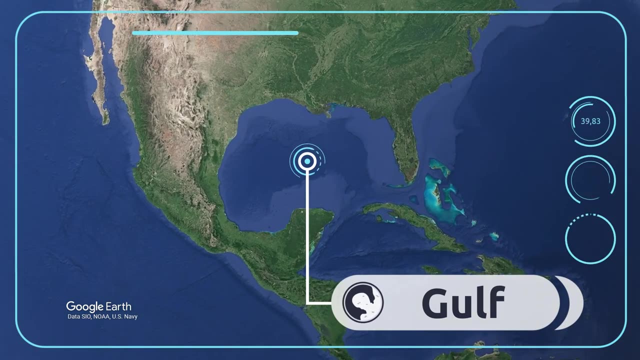 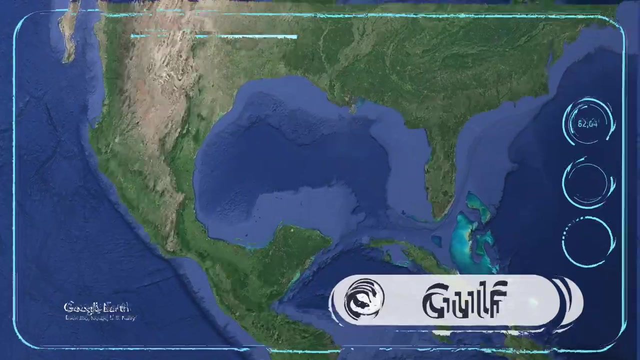 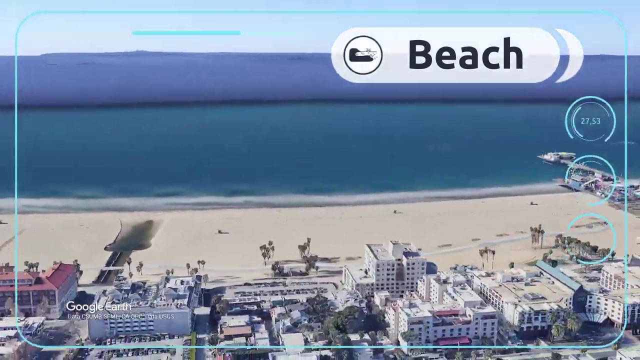 Cape Gulf. A gulf is part of the sea that extends into the land enclosed by two capes. Look, that's the Gulf of Mexico, Impressive Gulf Beach. A beach is an area of sand or pebbles near the shore of the sea, river or lake. 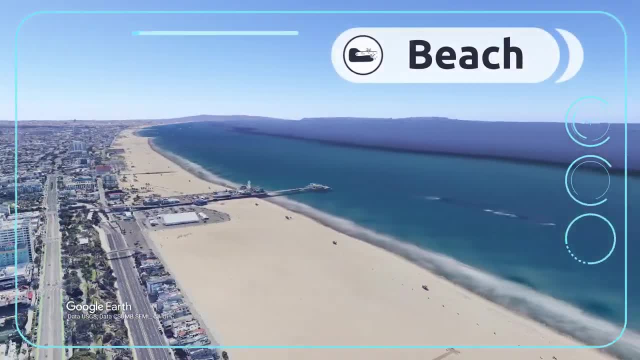 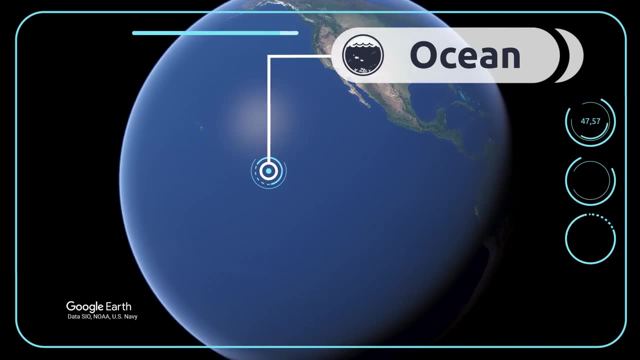 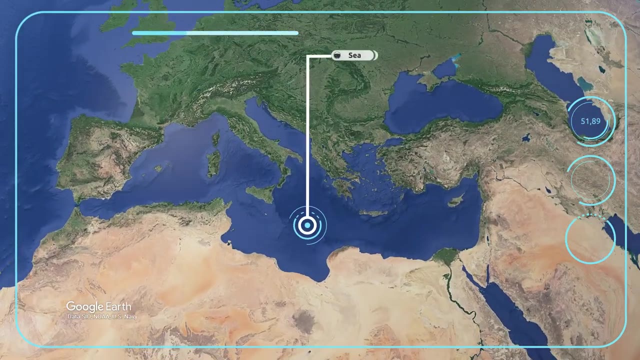 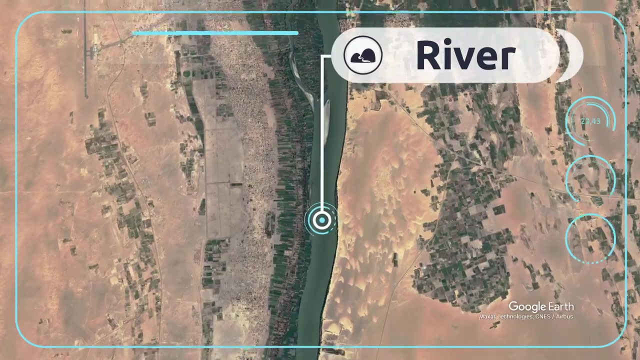 I love the beaches in Los Angeles Beach. Continents are surrounded by oceans and seas. This is the Pacific Ocean And the Mediterranean Sea. Let's continue our journey. River A river is a stream of water that may flow into the sea, a lake or another river. 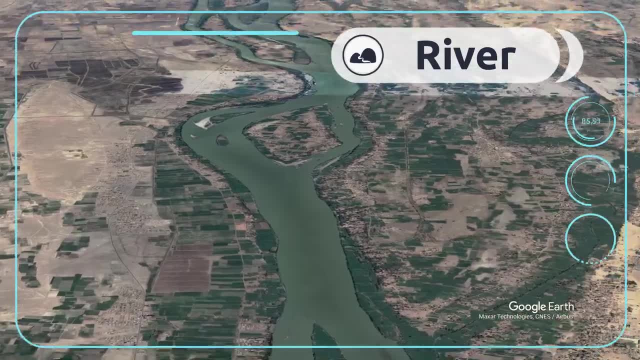 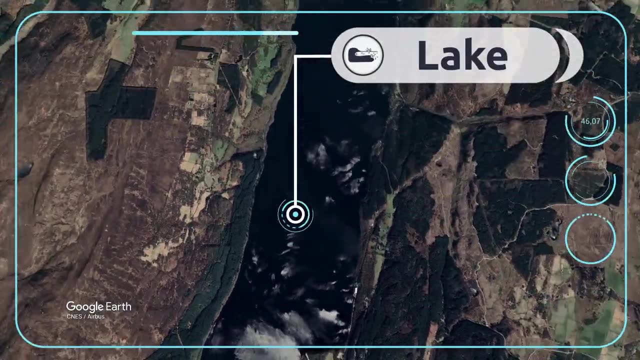 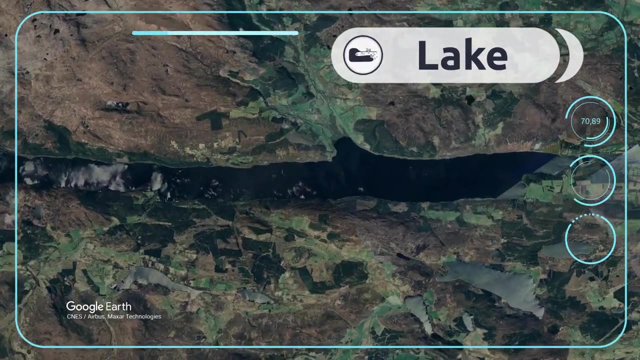 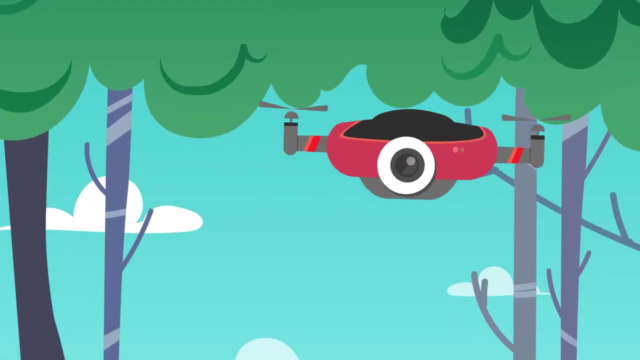 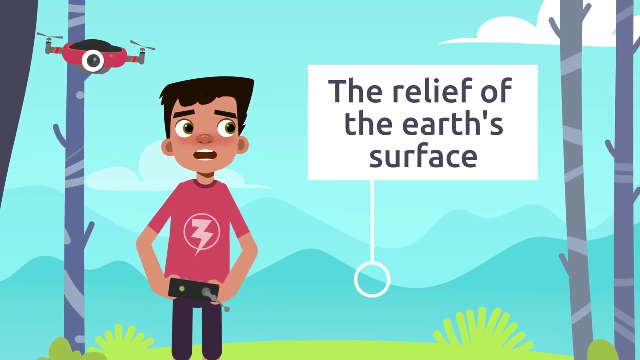 The Nile River is the longest in Africa River Lakes. A lake is a large inland area of fresh water. Let's fly to the Loch Ness Lake in Scotland Lakes. This has been a sensational journey. We've learned that the relief of the Earth's surface is the elevation changes in the landscape. 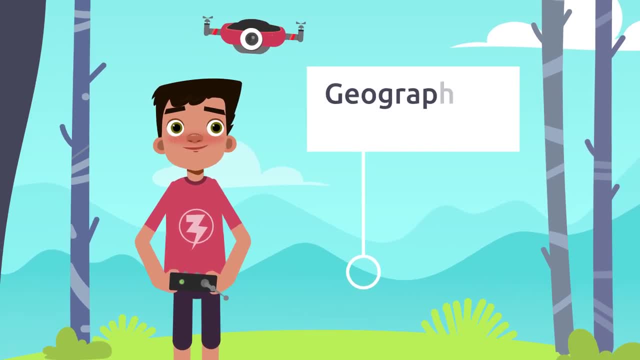 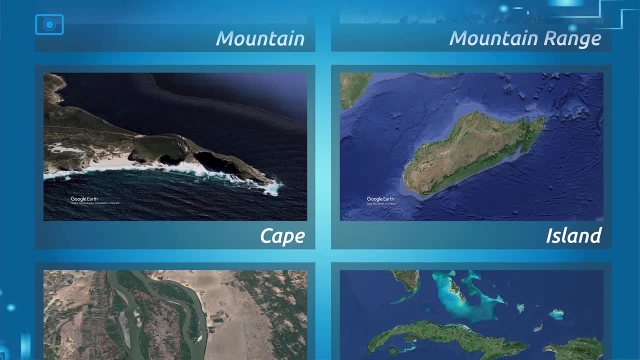 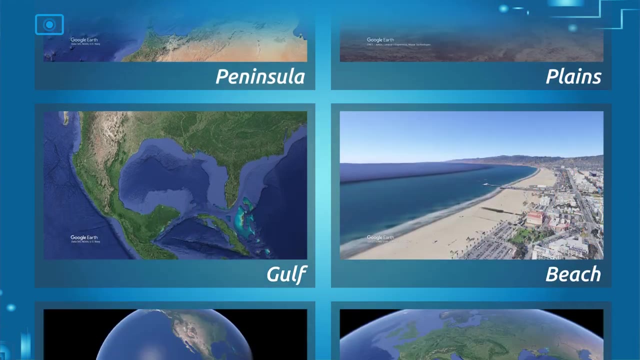 and that these elevation changes or landforms are called geographical features. Mountains, Mountain ranges, Mountains, mountains, mountains, Caves, capes, islands or rivers make up the Earth's relief. I've taken thousands of pictures and discovered some of the secret marbles of the Earth. 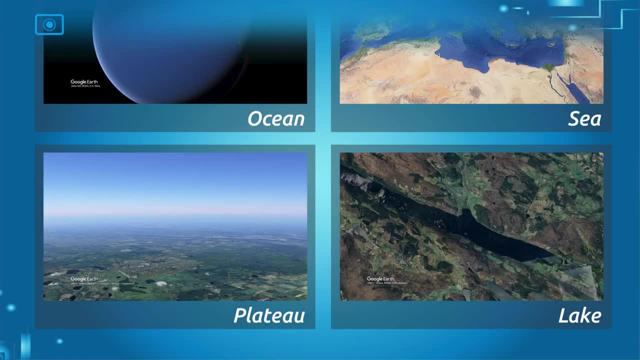 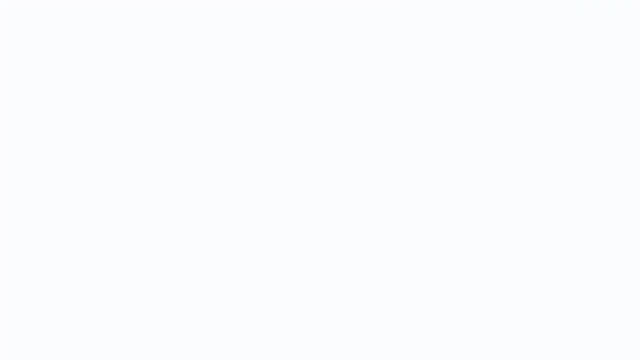 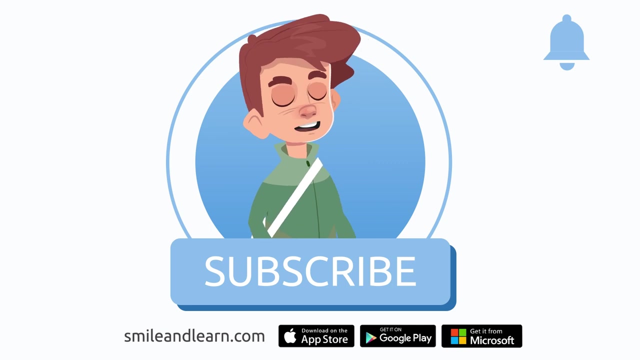 See you soon. friends, We've learned so much in just one video. Did you know there are many more videos? Imagine how much you could learn. Subscribe to the Smile and Learn educational channel to learn and have fun at the same time.